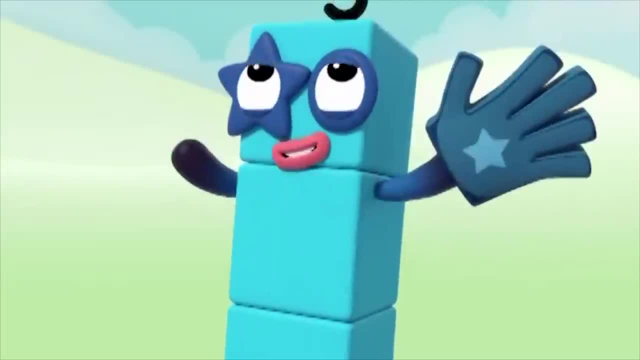 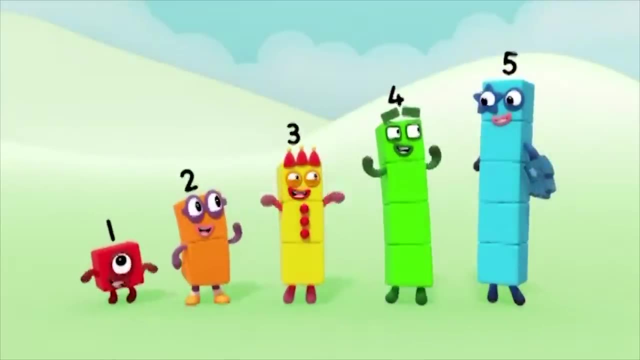 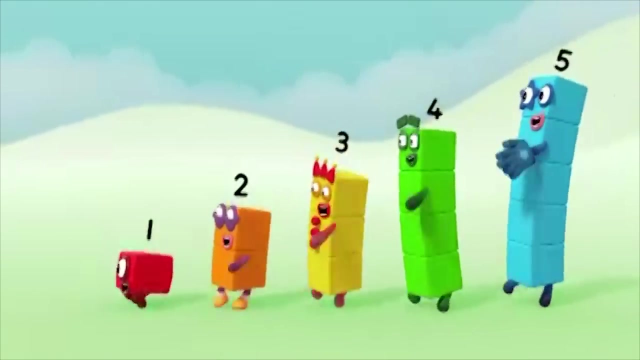 Pretend to be pirates, Discover a whole new world. Let's have an adventure. Hooray, Everybody ready. Off we go Off. we go on a big adventure. We don't know what the day will bring. Off we go on a big adventure. Ready, steady, sing. 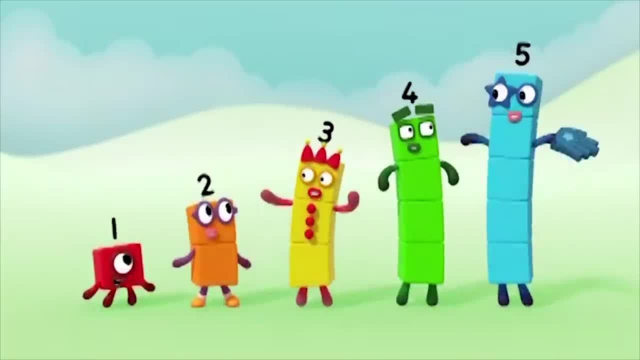 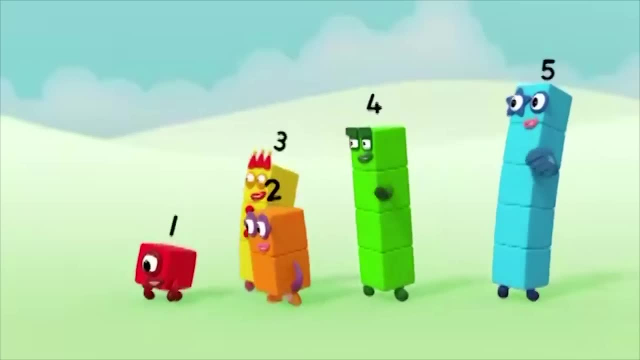 One, two, three, four, five. That sounds right. And off we go again. Off we go on a big adventure, We don't know what the day will bring. Off we go walking in the sunshine, Ready, steady, sing. Wait Too short, Can't see. 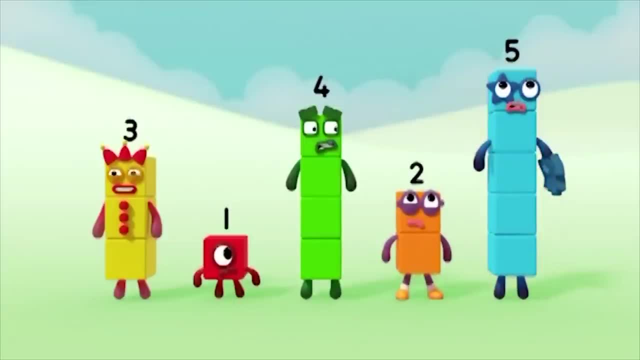 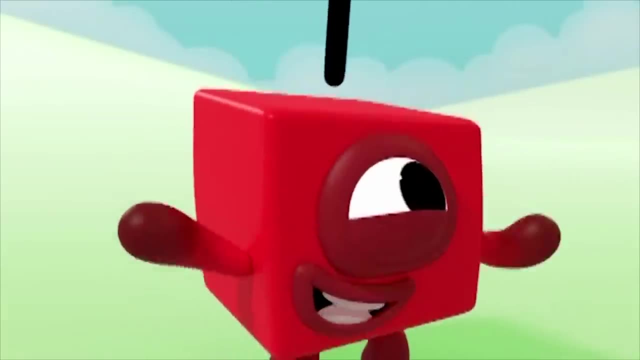 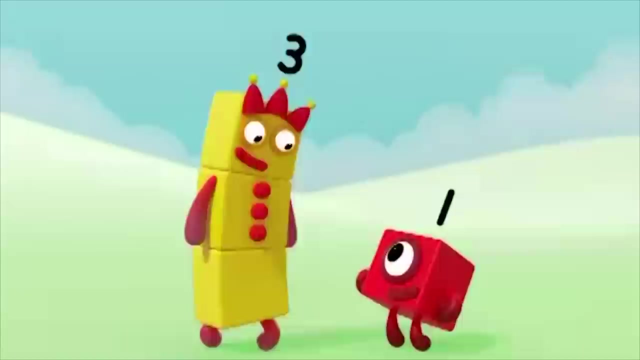 Three, one, four, five. That doesn't sound right. We're in the wrong order. I know what to do. Diddly, diddly do. Smallest that way, Biggest that way, This way Go, I'm bigger than you. 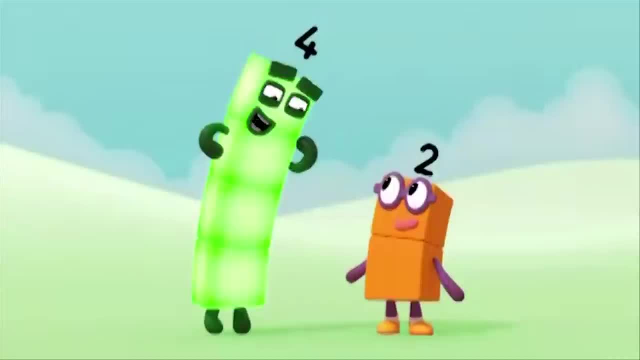 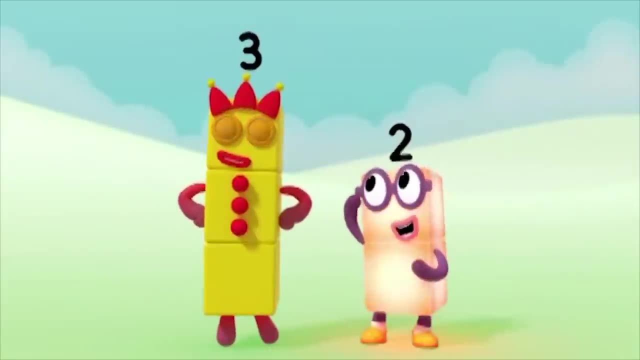 I'm smaller than you Diddly diddly do. I'm bigger than you. I'm smaller than you Diddly diddly do. I'm bigger than you. I'm smaller than you Diddly diddly do. 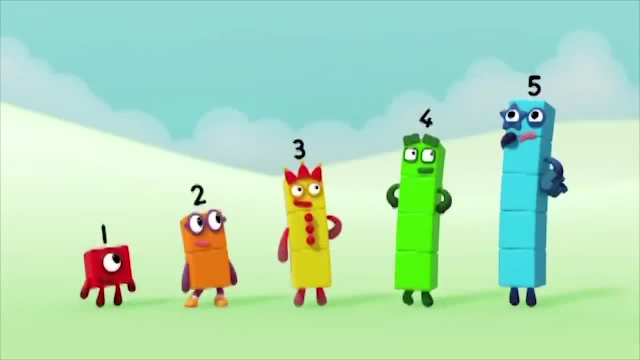 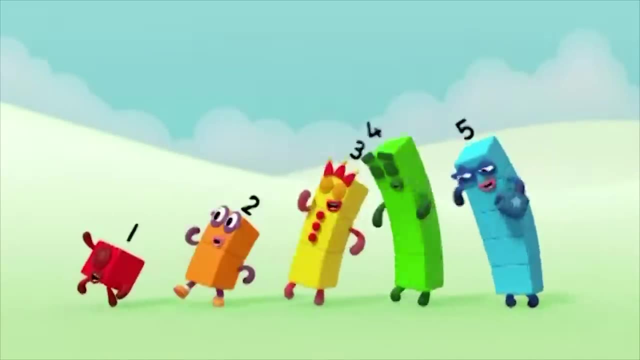 Are we all in order? Did we all do the right thing? Ready, steady, sing One, two, three, four, five. That sounds right. And off we go again, Off we go on a big adventure. We don't know what the day will bring. 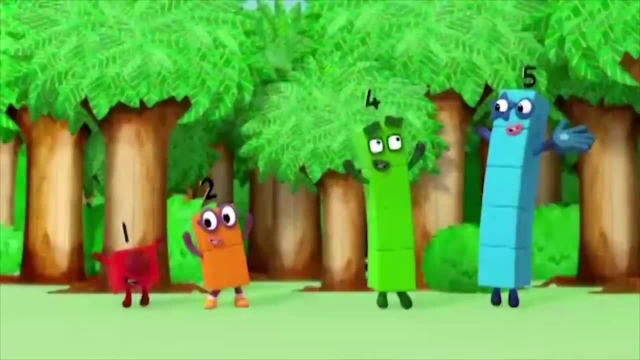 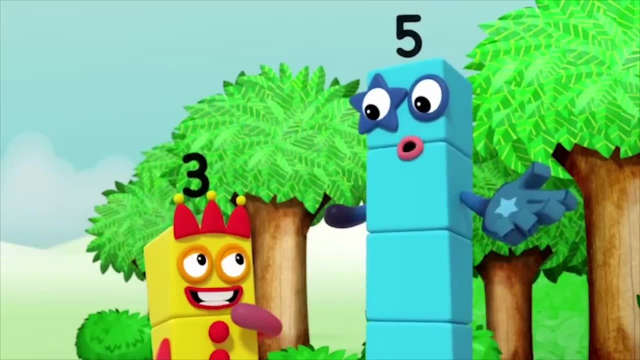 Off we go, running through the forest, Ready, steady, sing. You can count on us with an autobox Three. do you know how to count? Yes, of course. Look at a bunch of things, say some numbers and then say three. 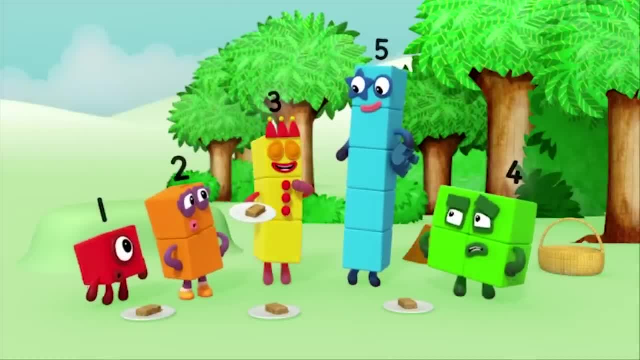 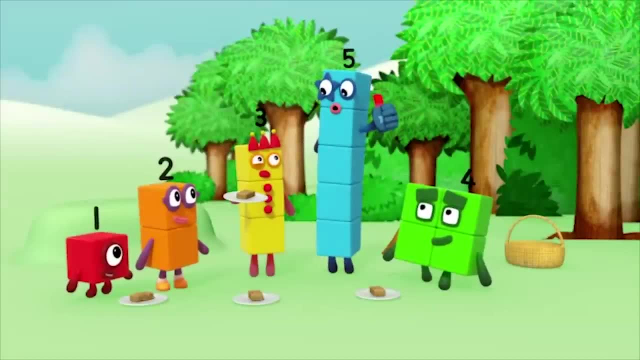 Because three's the best number. There's a little more to it than that three. There are some rules you have to follow. Rule one: count everything once. Try counting those flapjacks. It can help to put them in a line. 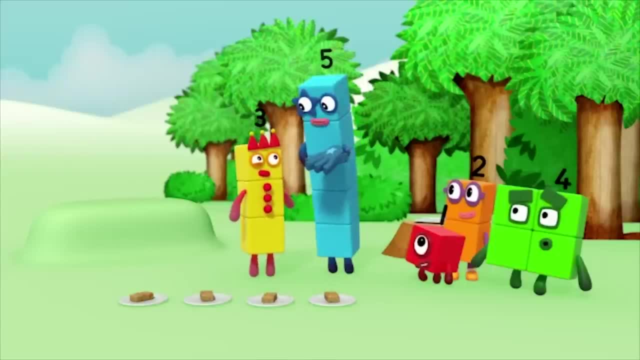 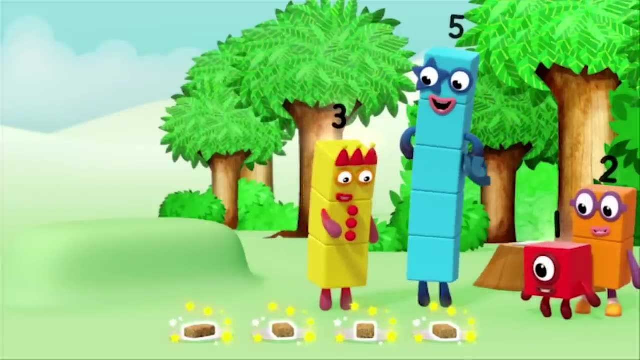 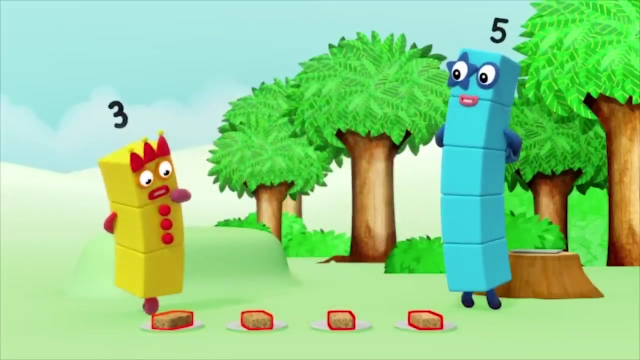 and to point at them one at a time, to make sure you don't miss any Or count the same one twice. One, two, three, four. Very good, Four, three, two, one, Wait one. That's not right. 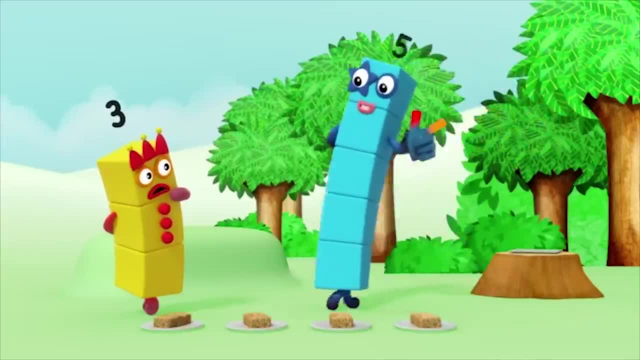 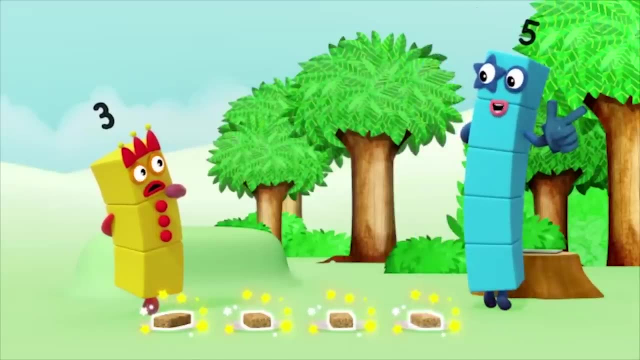 Rule two: Say the number again, The number's in the right order. If you don't say them in the right order- one, two, three, four- you won't know how many there are. Oh, One, two, three, four. 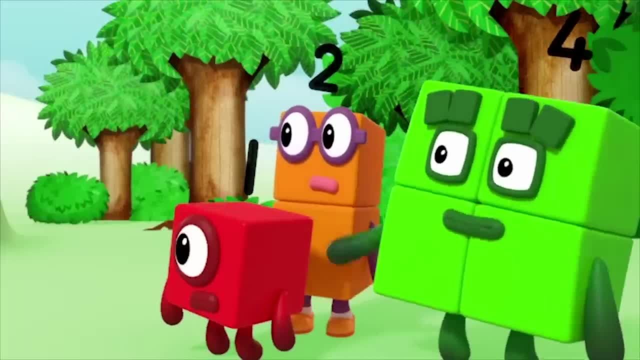 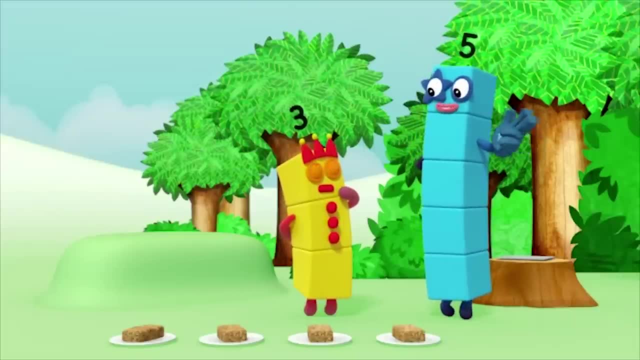 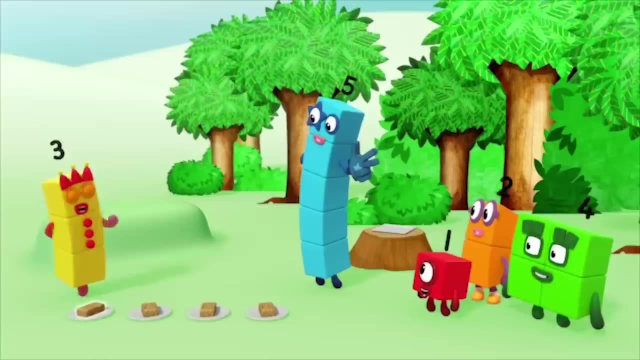 Three flapjacks. Oh, we've been here before. Rule three: The last number is how many. When you reach the last thing to count, the last number you say tells you how many there are. Try, You can do it. Go on. 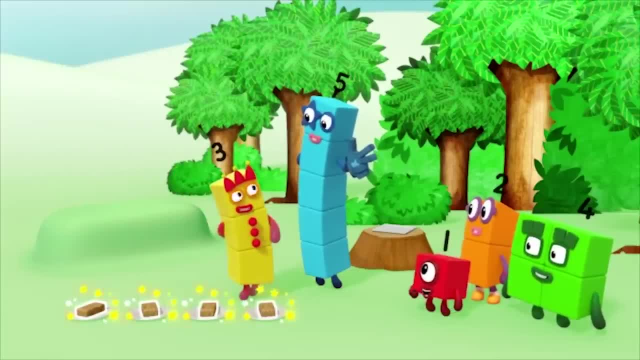 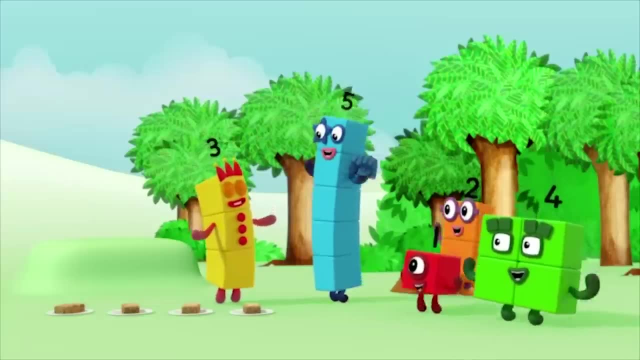 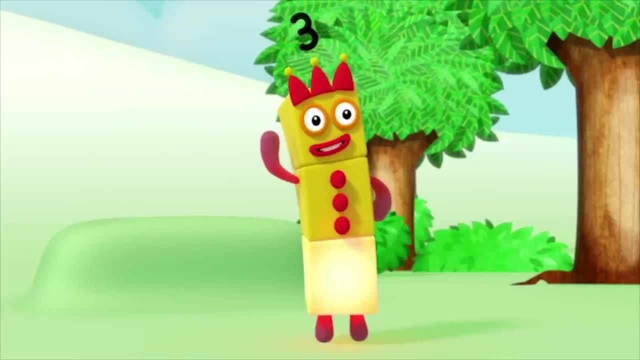 One, two, three, four. That's the last flapjack. So four flapjacks, That's right. Yeah, I did it. I know how to count. One count everything once. Two say the numbers in the right order. 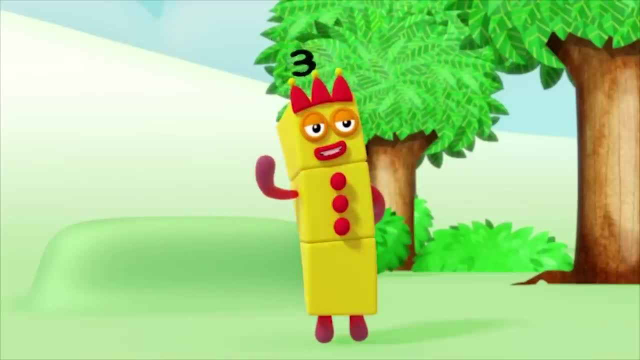 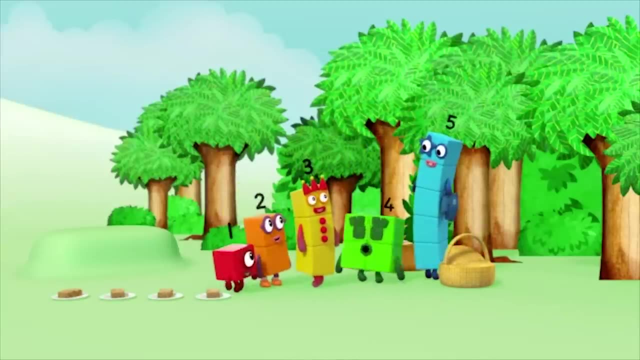 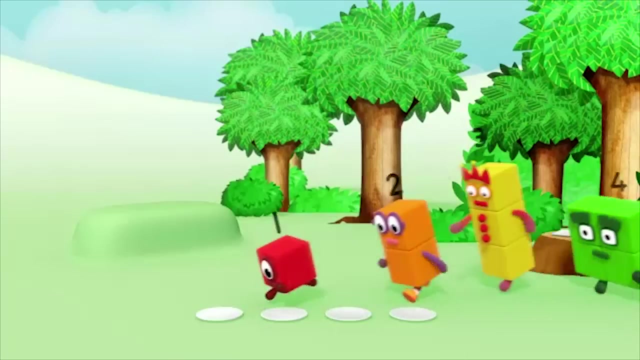 Three. the last number is how many? Three rules of counting. All right, Let's celebrate with flapjacks. I've packed an extra one for you: five. Hang on, It's gone. Oh, Oh, Oh, Oh Oh. 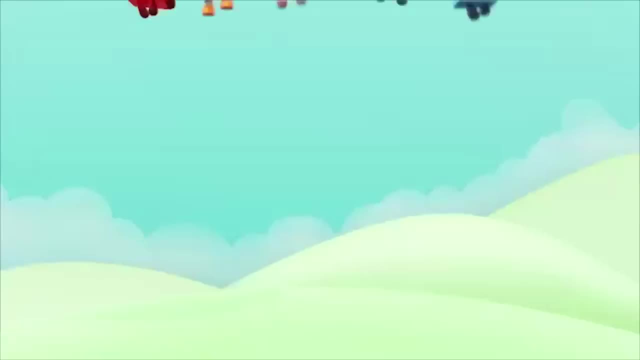 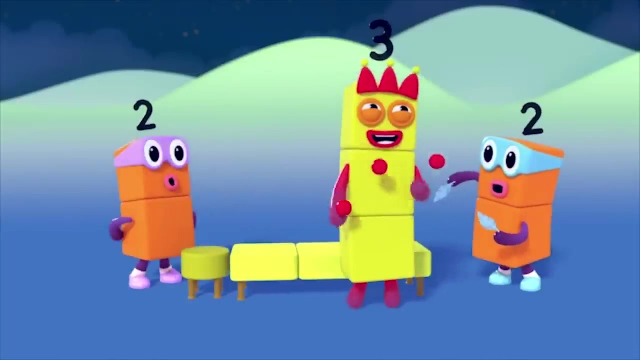 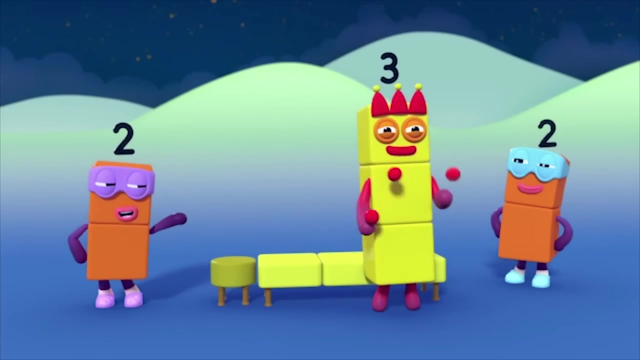 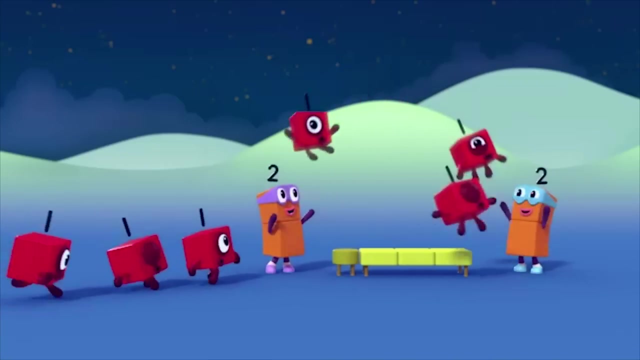 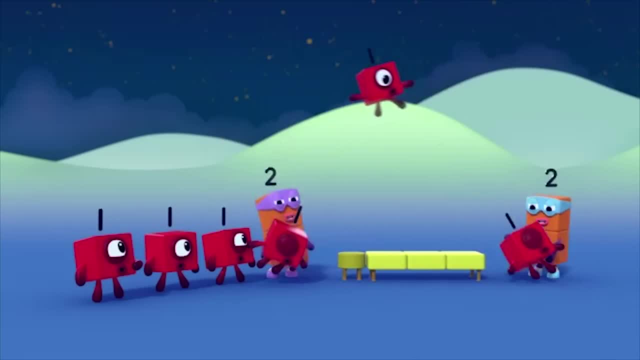 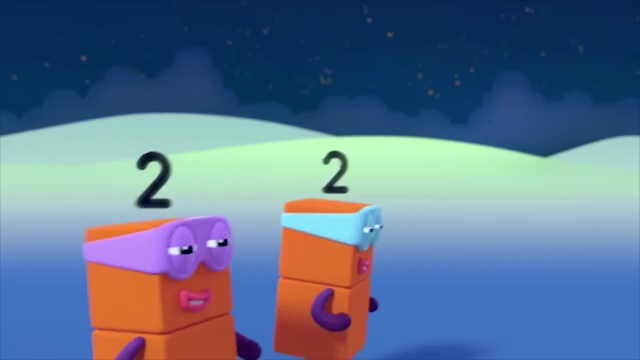 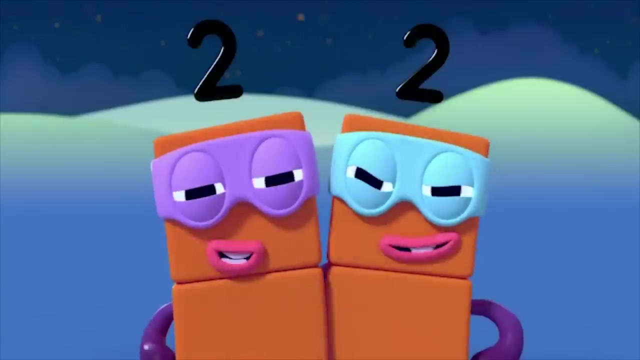 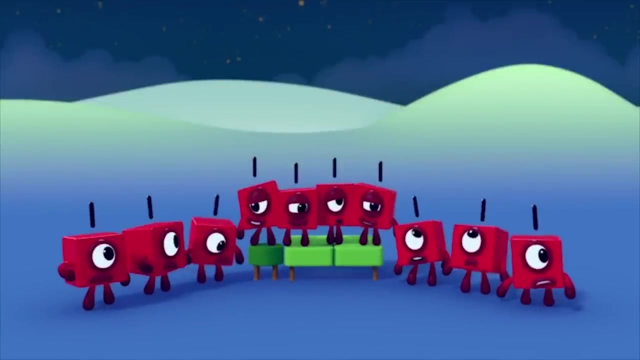 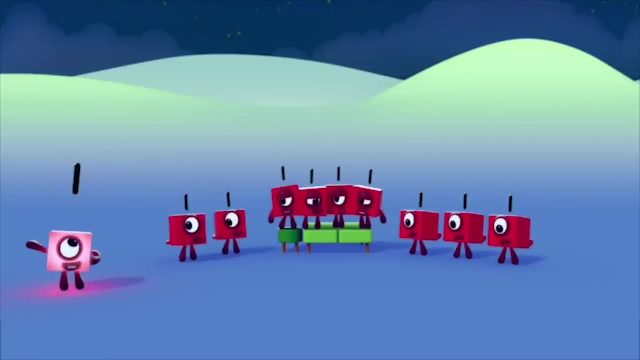 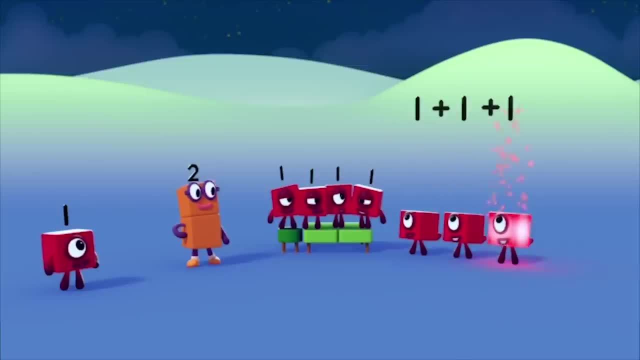 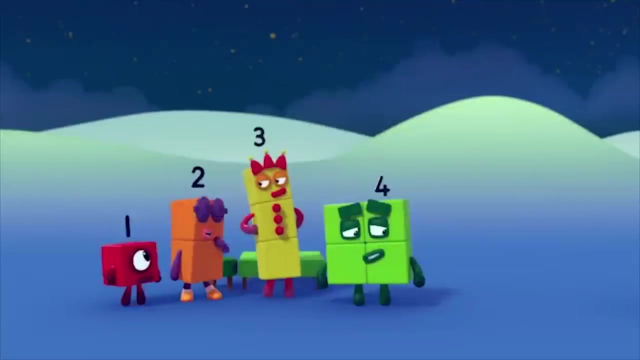 One plus one plus one equals three. Three is three ones. One plus one plus one plus one equals four. Four is four ones. Where are they? Where did those terrible twos go? Don't look at me. What's all of the noise? 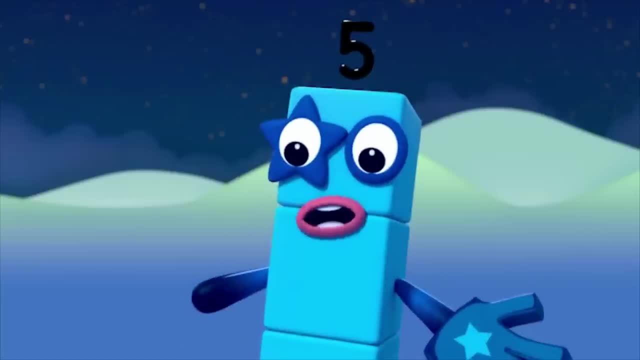 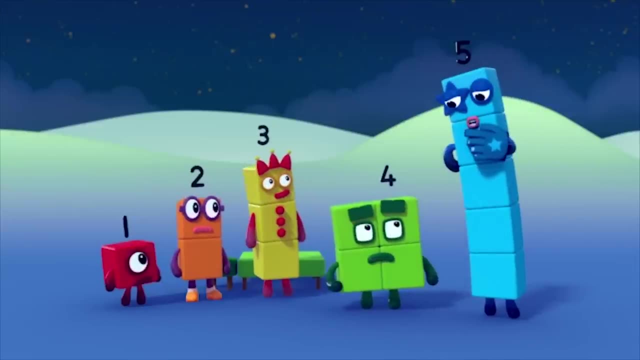 The terrible twos are playing. They're playing tricks on us, And where are they now? I have to be square with you. They made me. What did they make you? You can tell us Four. No, they made me. 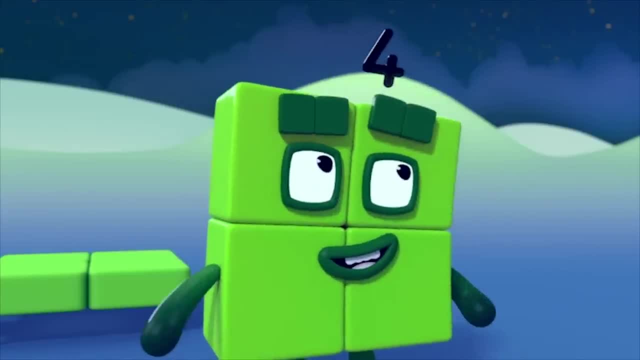 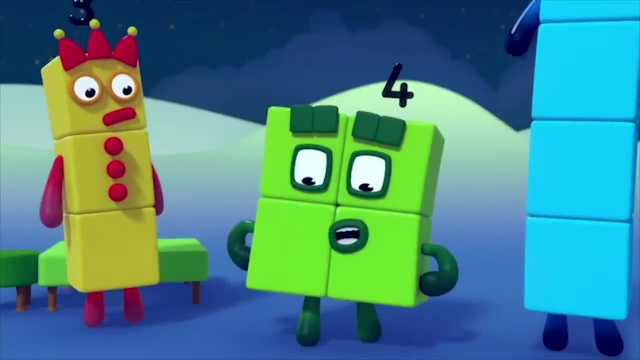 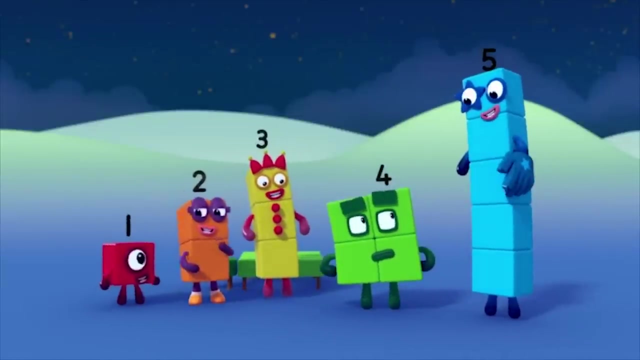 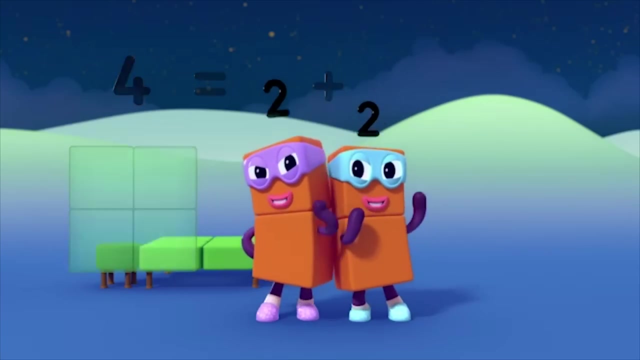 Well, I made them, Then they made me. Huh, I'm the terrible twos, I'm four lots of one, But I'm also two lots of two. You're funny, Very funny, Charlie. Yes, the одной и Всё. 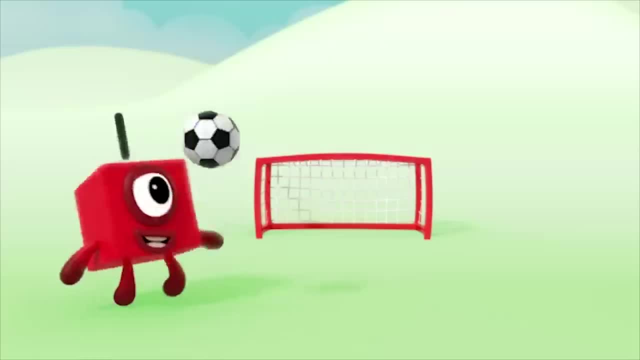 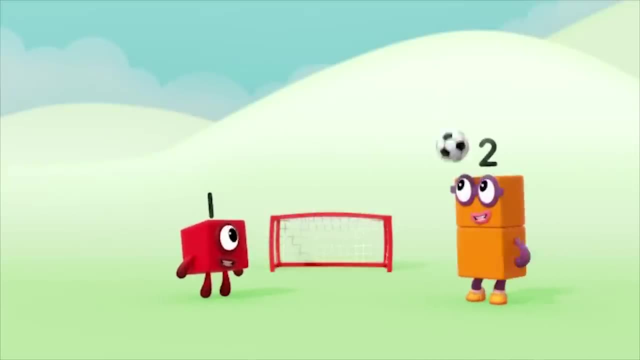 You know somebody who turned out to be Blue, Look at questions and what to do. Well, either you have to eat this for your favourite cuisine or Theman 차 realistically gave you a discount. Academy is closed. C'est Eddy's turn. 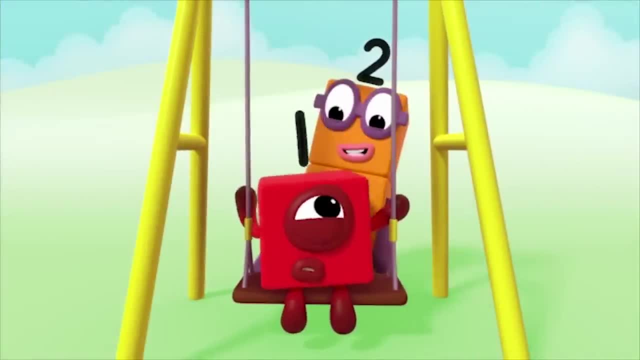 The internet is off. You can sleep. if you lie there, Go, C'est Eddy's turn. if you lie down. Yes, the internet is off. Yes, Theman 차 ridiculously lied to me: The swings are boring, Cos you need a friend to give you a push. 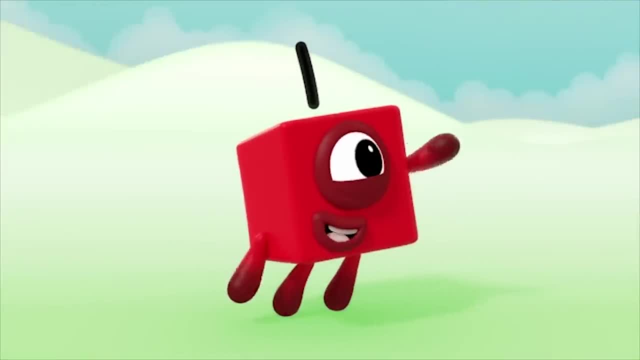 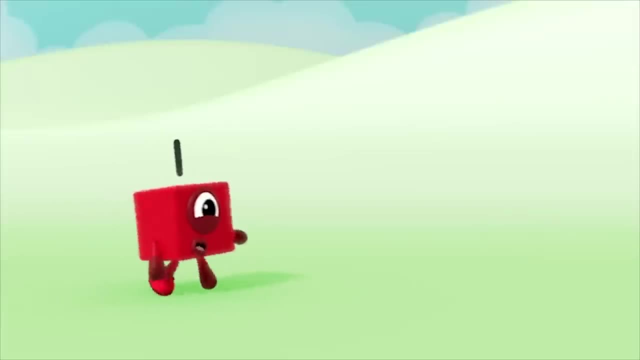 With one you can get a bird in the hand. Oh look, there's two in the bush. One shoe just won't do. You'll end up all lopsided. One, two, two shoes You can use to dance like I did. One wing tied with string. 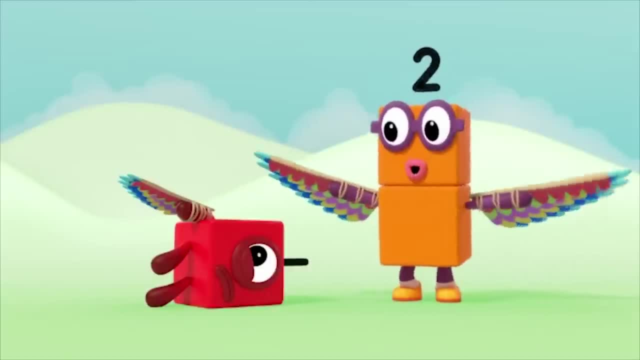 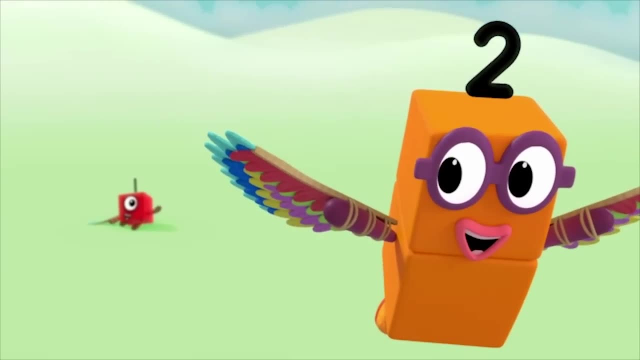 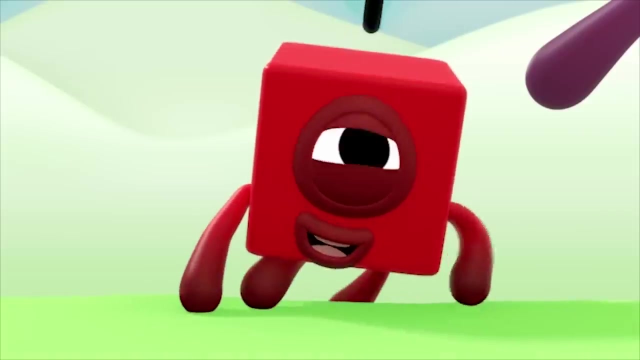 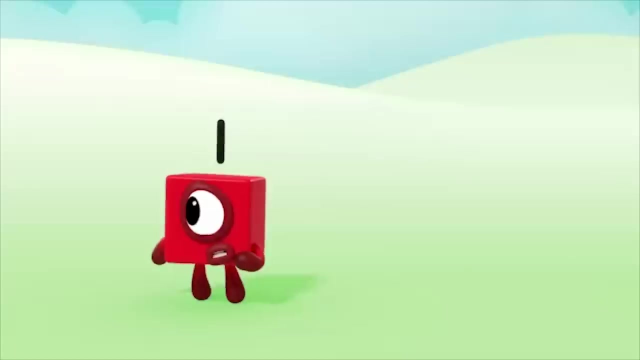 No point even trying. One, two, two wings And zing, you'll soon be flying. With two, you can get a leg up. With two, you can offer a hand. With two, you'll never be fed up, Cos there's always someone to understand. With two, you won't. 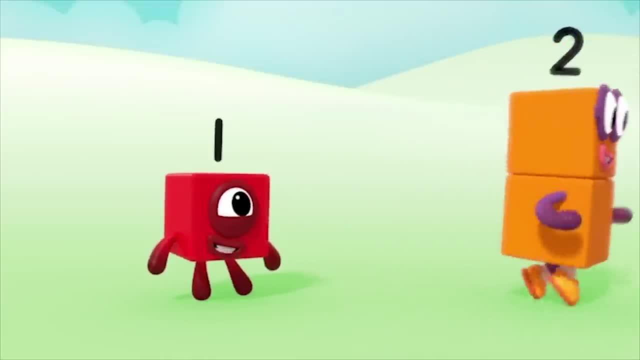 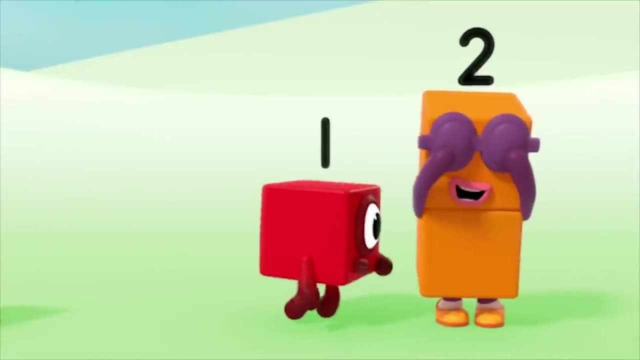 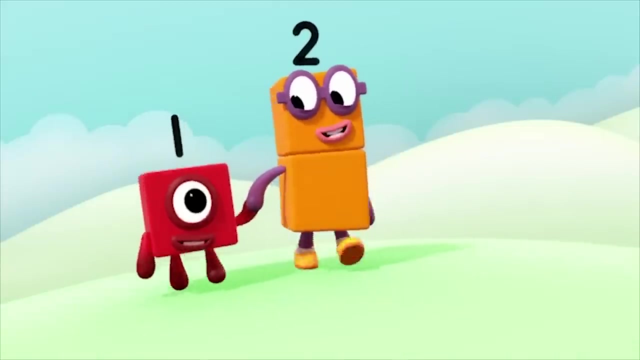 Be lonely And you're never gonna have to pretend. With two, you can play Hide and seek. With two, you can find a best friend, Cos everything is better with two, The two of us together, Just me, and you Imagine all the crazy things we can do With two. with two, 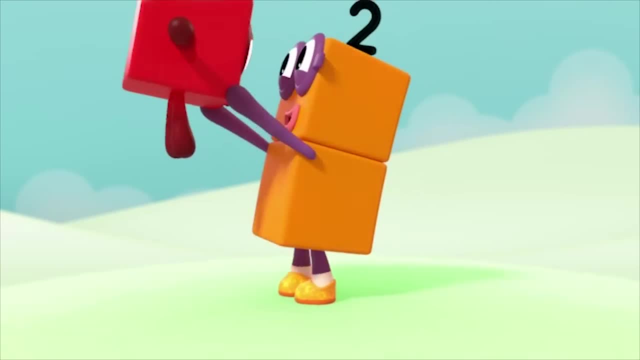 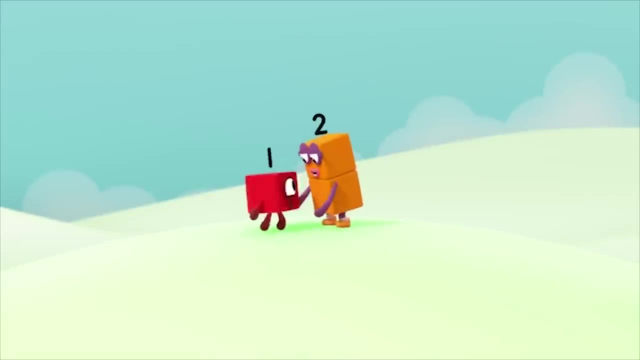 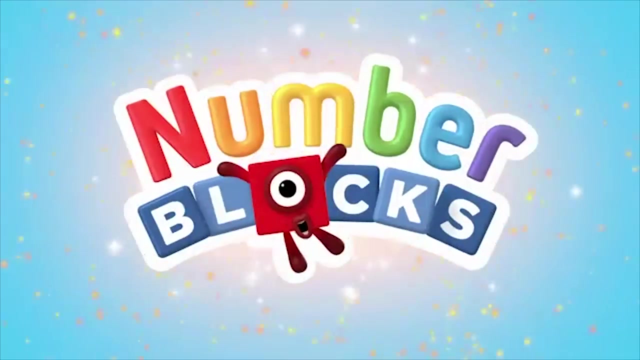 With you and me and me And you With two, we'll see what fun can be With you and me, and me and you, And all the things we can do With two. Best friend, Best friend, You can count on us with another box Apple on top. Don't let it drop. 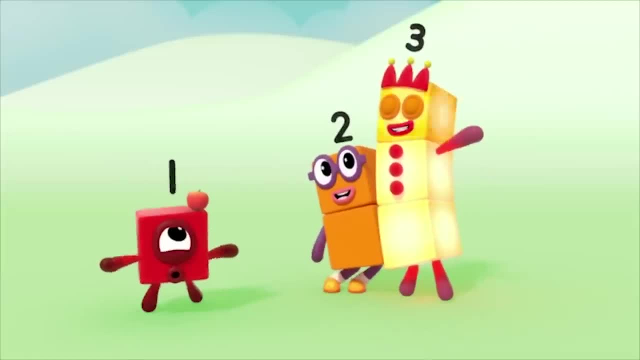 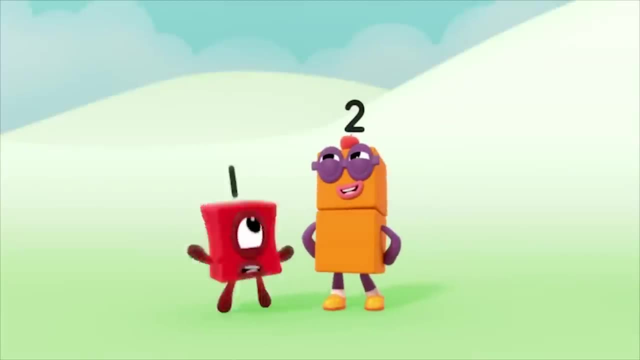 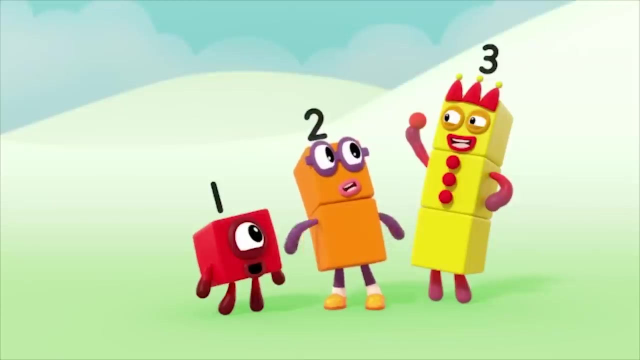 Now Try and swap. Hey, I can't reach. I'm smaller than you. I'm the smallest number, Then I'm bound to win. I'm bigger than you. Oops, silly me. I'm bigger than one, but smaller than three. I'm bigger than both of you. 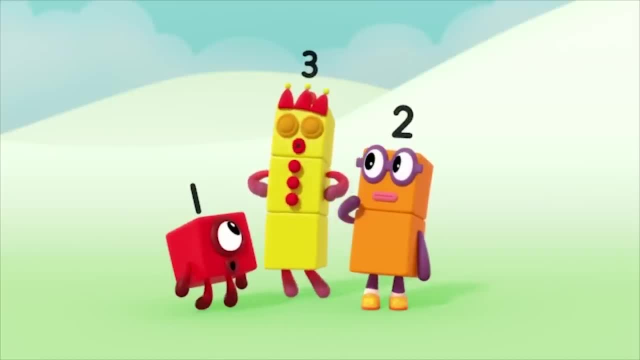 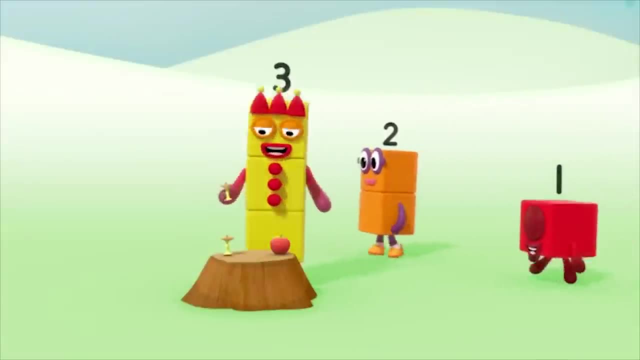 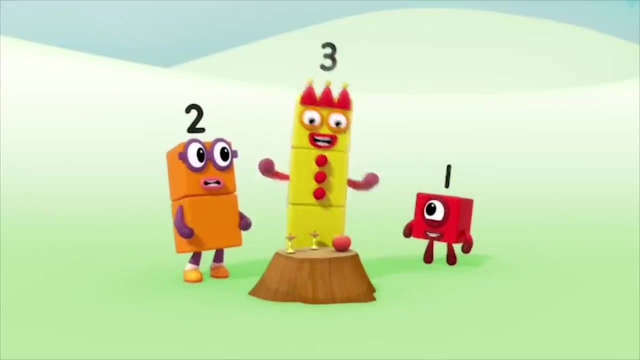 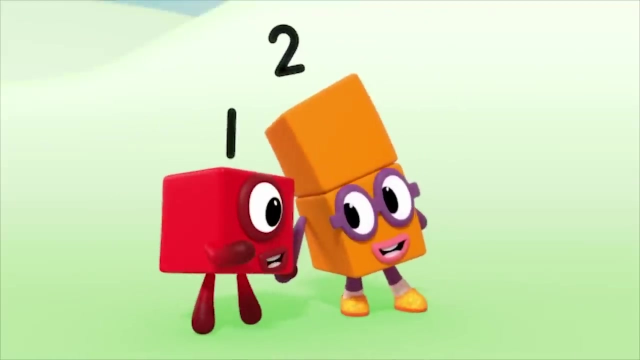 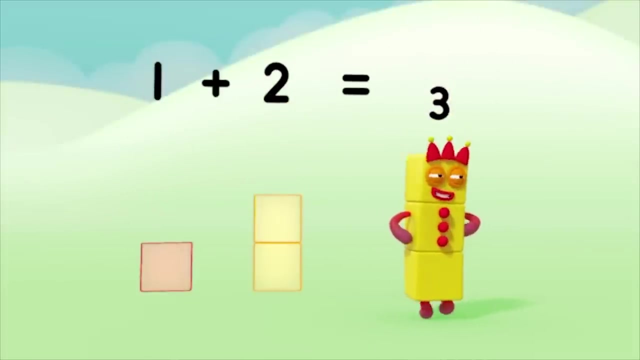 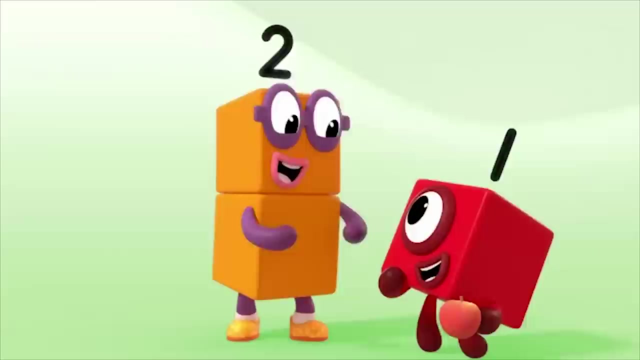 I'm the biggest, So I guess I win again. One, two, three, Two apples gone, One apple left. Surprise, It's the final game. The biggest surprise wins: One plus two equals three. Three. One, two, three, Three equals Two plus one. Wow, But how. 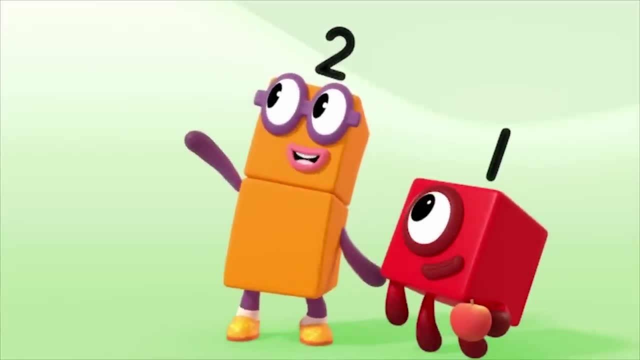 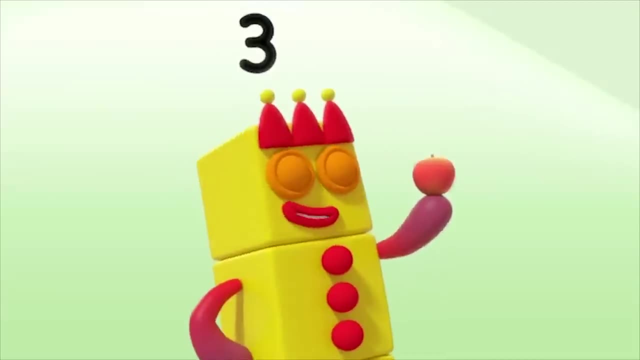 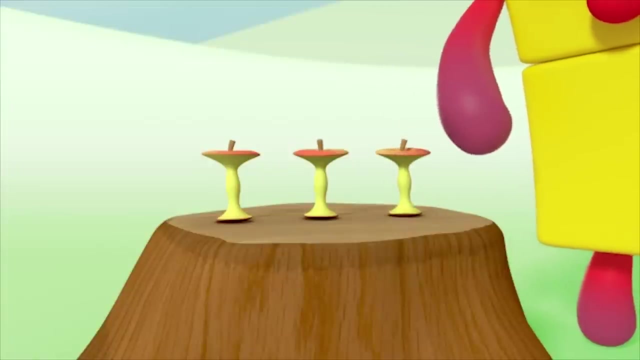 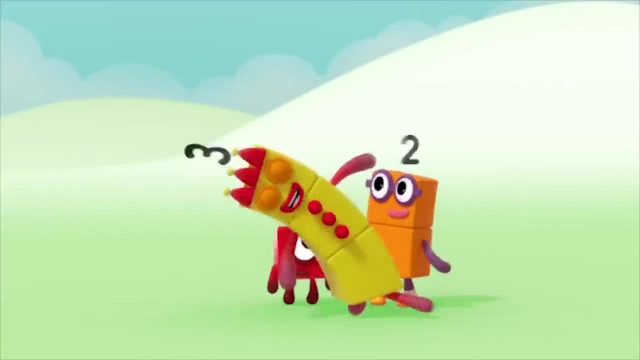 Very good, You win best. surprise Three, One, two, three, All for me. Oh, that was the last one. Oh, that was the last one. Oh, that was the last one, That was the last one. Aww, Don't be sad, Don't be mad.